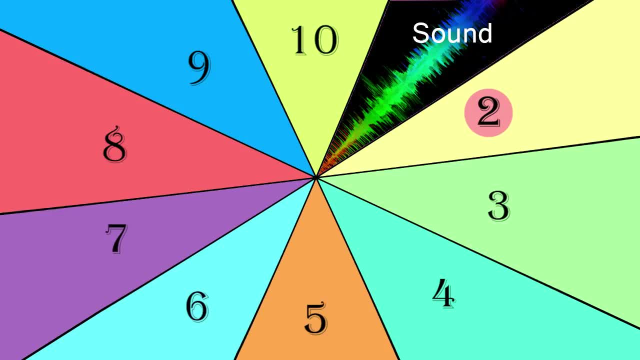 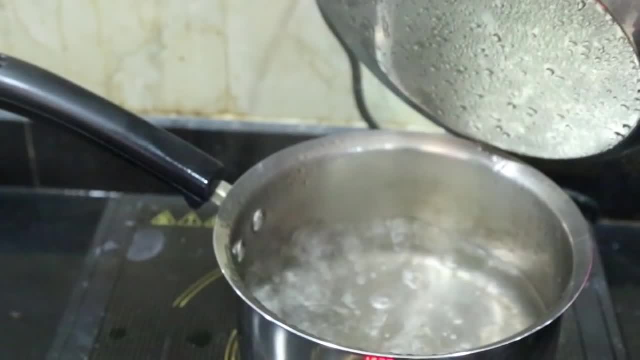 before we define what physics is in the end To have a cup of coffee, we boil water. After turning on the stove, we notice that the water is hot enough when it starts boiling and when we see steam. This gradual rise in temperature that causes the water to bubble and later change to steam is called heat. 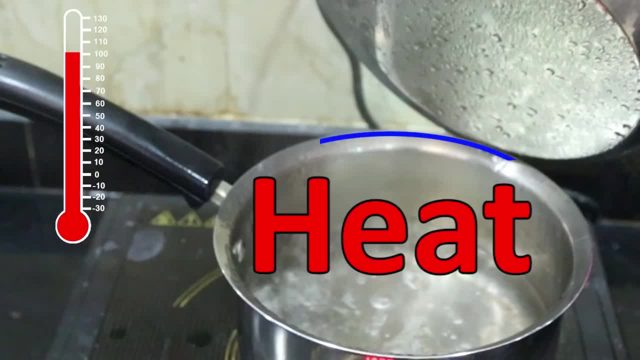 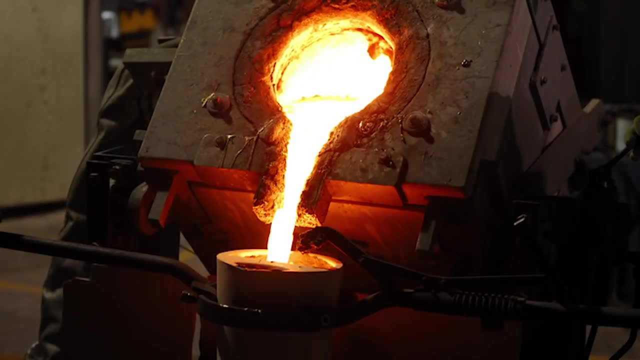 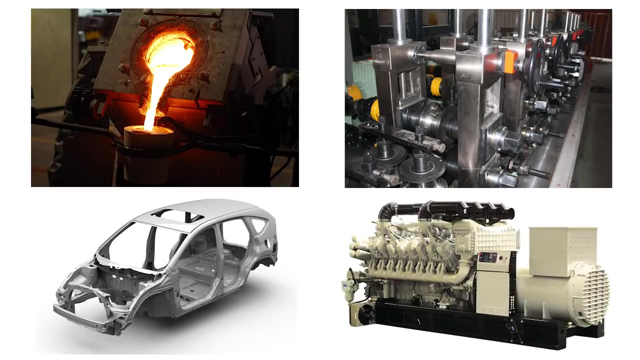 Thus we get hot water by heating that is, increasing the temperature of water. Heat is used in the industry to melt metal and make various types of heavy-duty machinery like automobiles and generators. It is also used in household appliances like the electric or steam iron. 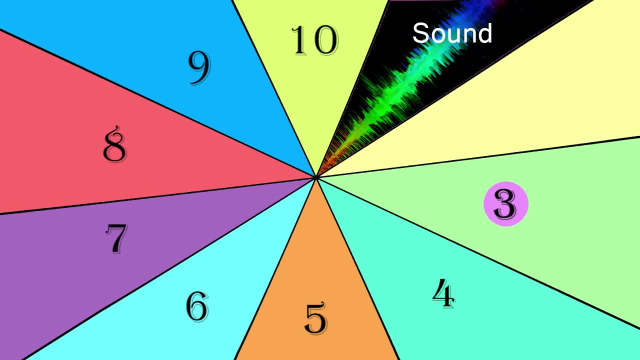 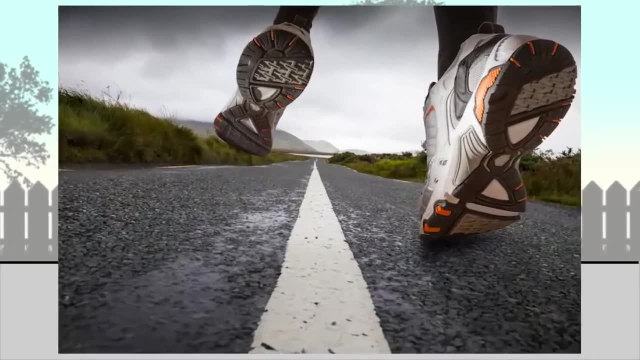 Heat and its properties is an important topic of physics as well. While we take a walk in the park on a tar road, we have a good grip without slipping because of a sort of roughness or resistance between the soles of our shoes and the surface. 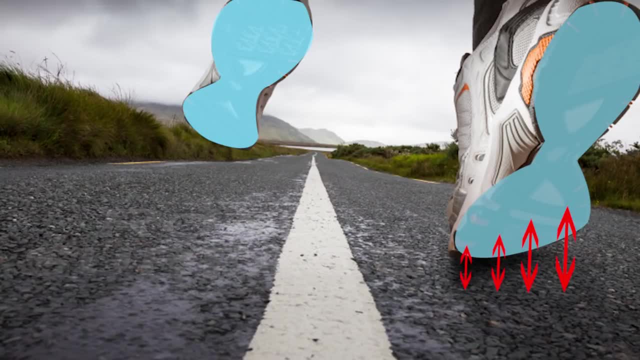 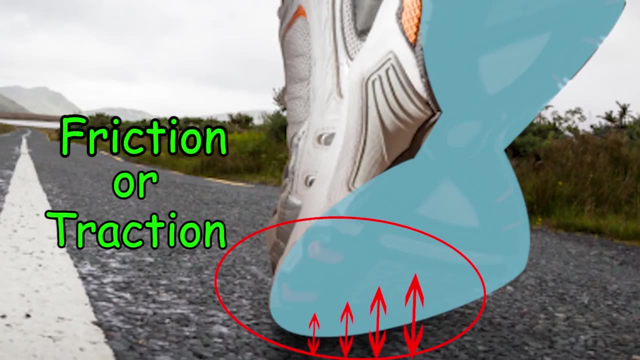 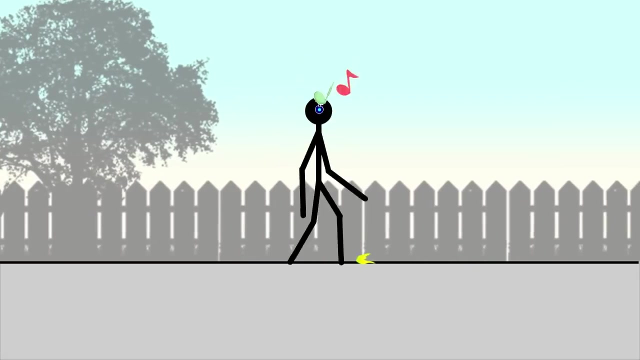 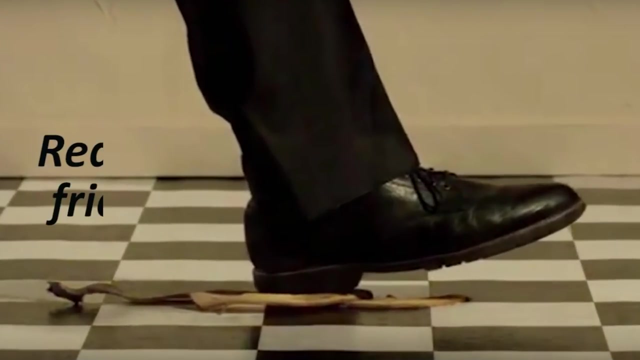 This resistance that's responsible for grip is called friction or traction. But say, if we're busy on our cell phones or waving at our friends and we do not notice a banana peel in front of us, What makes us fall? Well, apart from our absent-mindedness, it is due to the reduced friction between our shoes and the road because of the slippery banana peel. 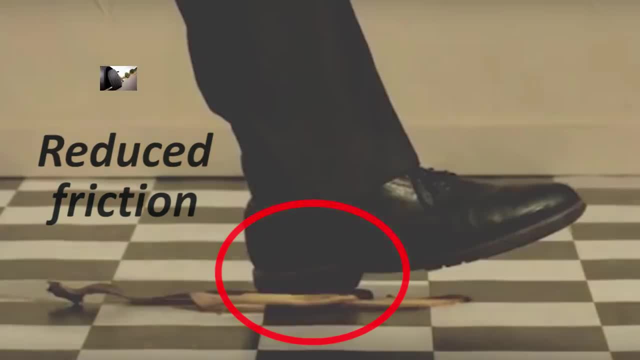 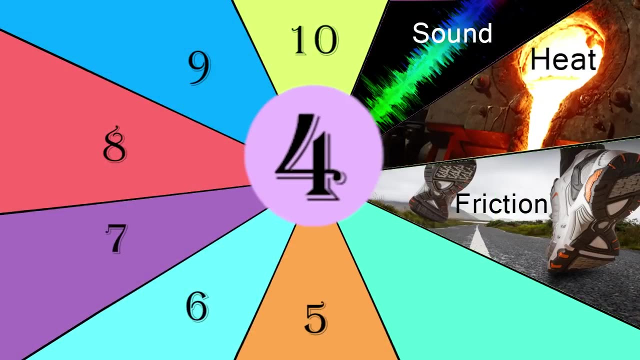 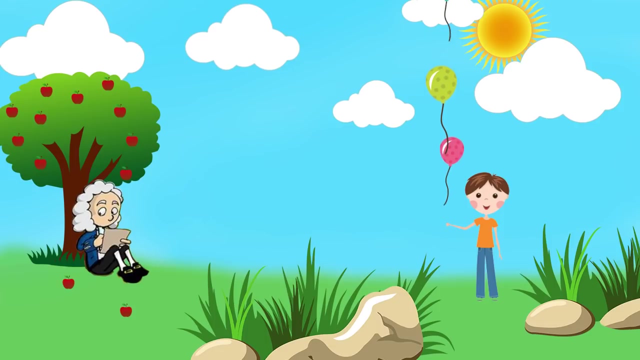 Friction, which is an important factor in the making of tyres, is also explained by physics. We have all observed apples falling from a tree or balloons floating away in air. How is this possible? The apples fall down while the balloons float up? 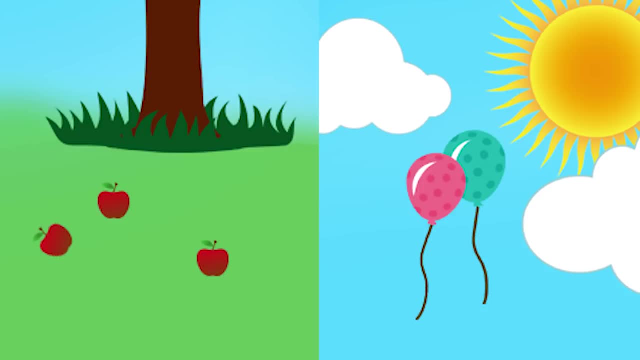 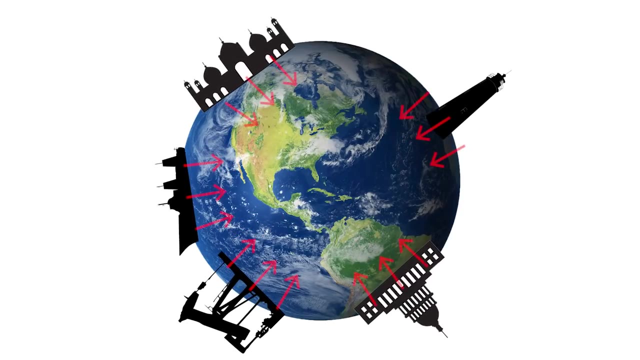 This is nothing to be puzzled about. The answer is simple. Our earth has a kind of a pull that draws every object to its surface. This pull is called gravity or gravitational force, which keeps every object grounded to the surface of the earth and prevents them from floating away. 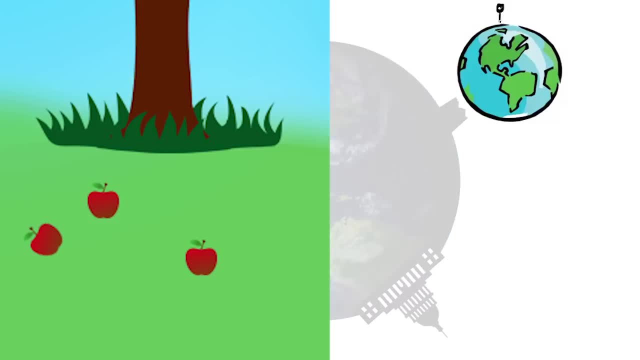 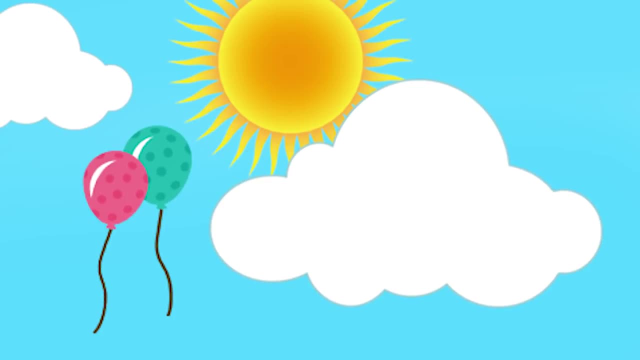 This is why apples fall to the ground and why people or objects on the underside of the earth do not fall into space. So why did the balloon float away and not fall to the ground Again? it's no big deal, We know. the air is light. 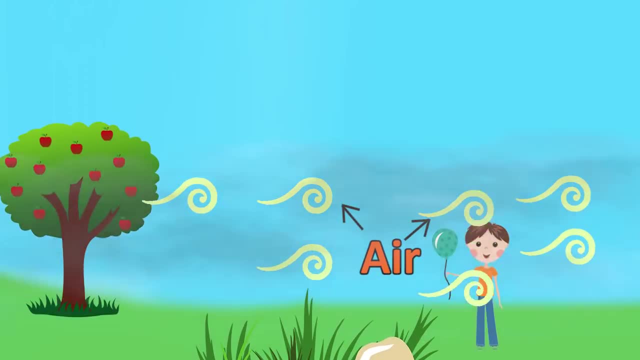 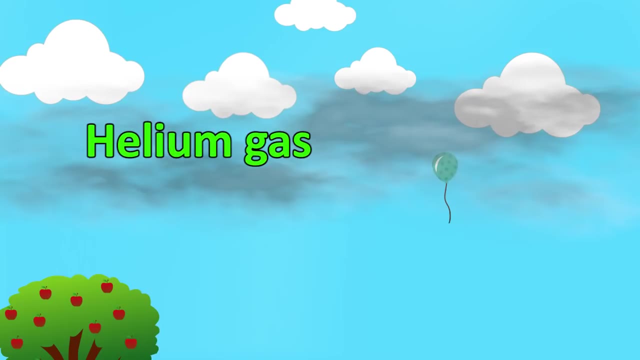 So imagine something which is lighter than air, like, say, helium gas filled into the balloon. Because it is light, it rises to a level higher than air and thus works against gravity, which now cannot keep the balloon grounded. Gravity is studied to a great extent by astronauts to mimic conditions in outer space. 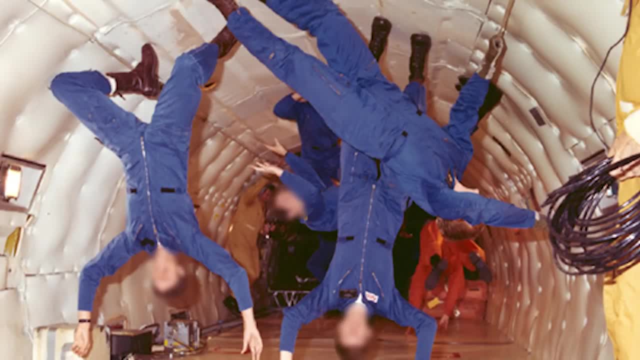 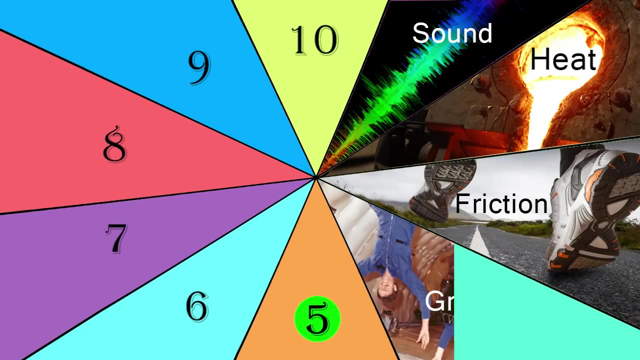 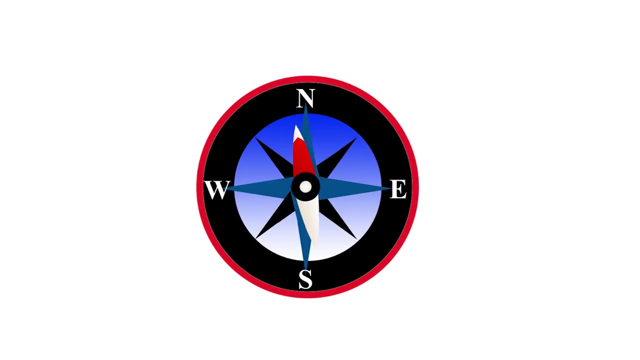 In fact, gravity is the very event that was studied by Sir Isaac Newton, who is now considered one of the fathers of physics. When we use a compass, we notice that the direction of the needle is constant. That is, the needle points in only one direction – north. 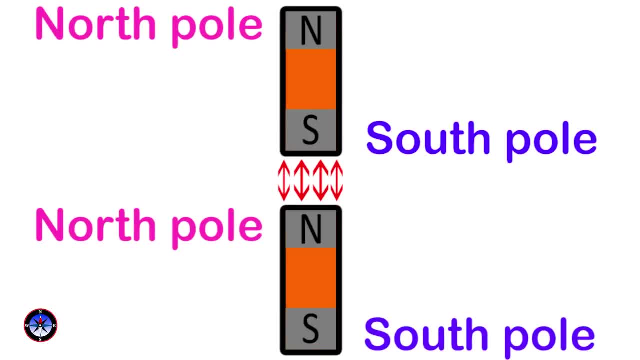 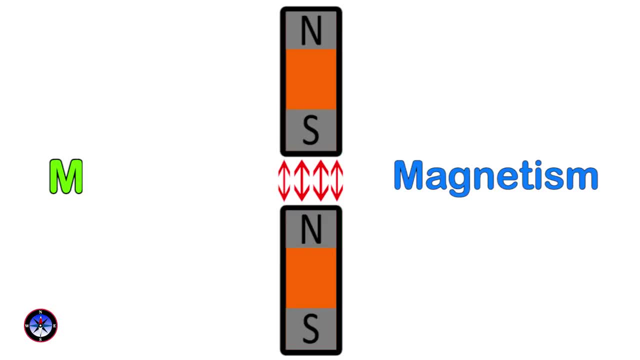 This is because of a force of attraction between two oppositely charged ends called magnetism. All materials that follow magnetism can be termed as magnets. Did you know that, apart from being just a planet, our earth is actually one big giant magnet? 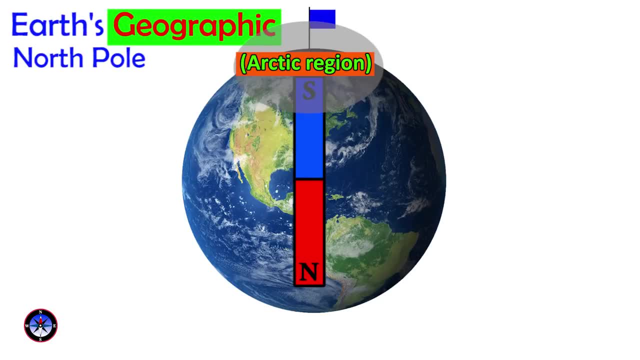 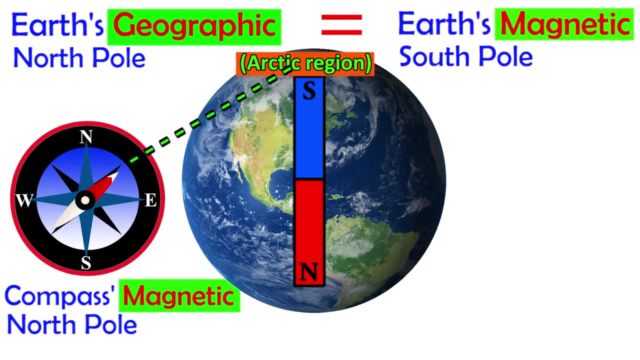 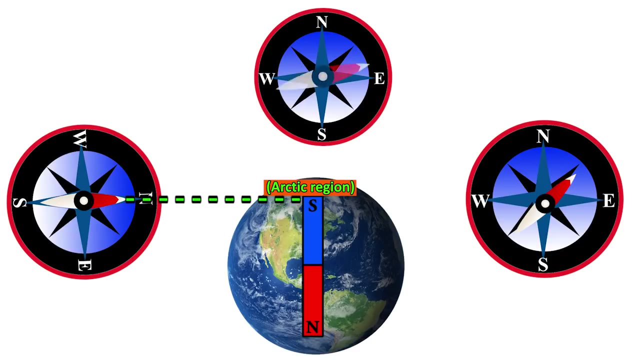 The geographic north pole of the earth, that is, the arctic region, is actually the magnetic south pole, which attracts the magnetic north pole of the compass. This is why the compass always points north, no matter where it is. We all know, opposites attract, don't we? 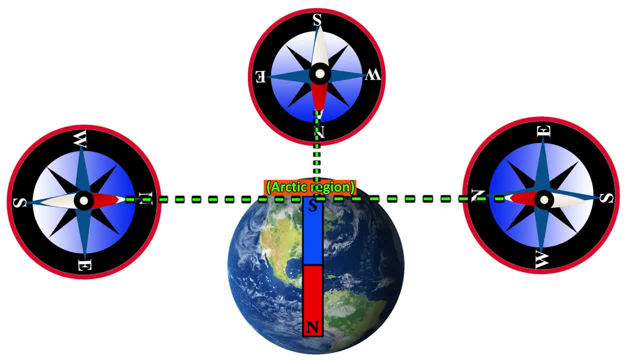 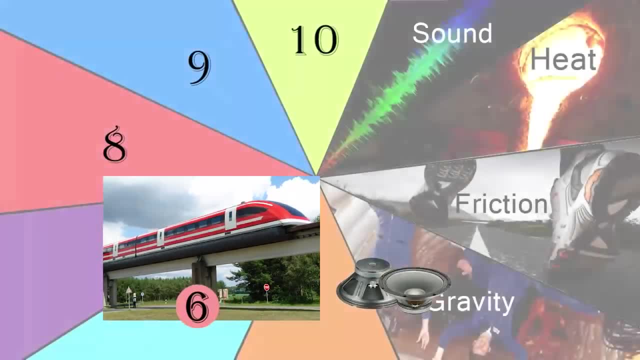 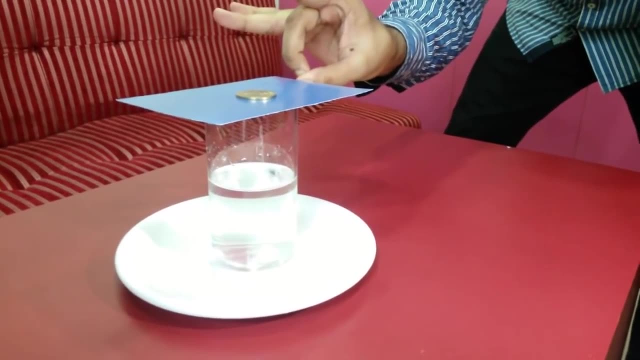 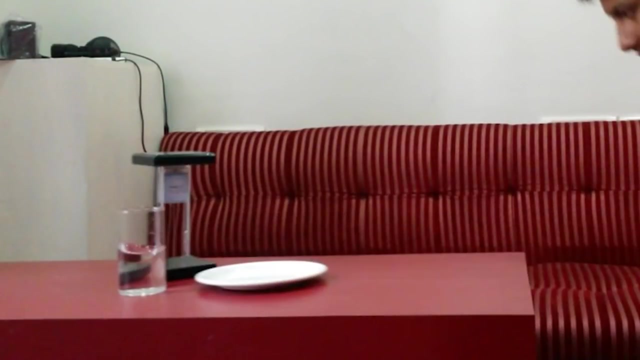 Physics looks into the property of magnetism, which is used in modes of transport like the metro, trains and in parts of electronic speakers. We would have all seen or done at least a few of these tricks. So what makes objects remain still or maintain its position even if there is a pull or tug on it? 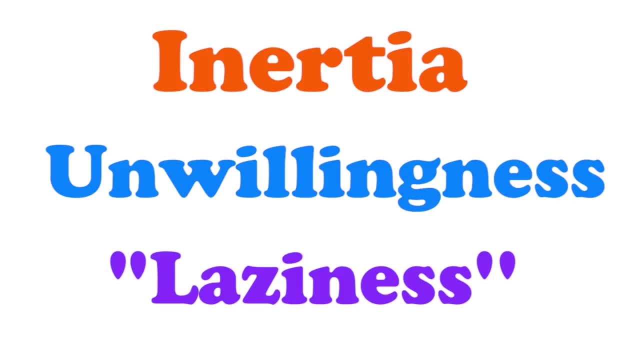 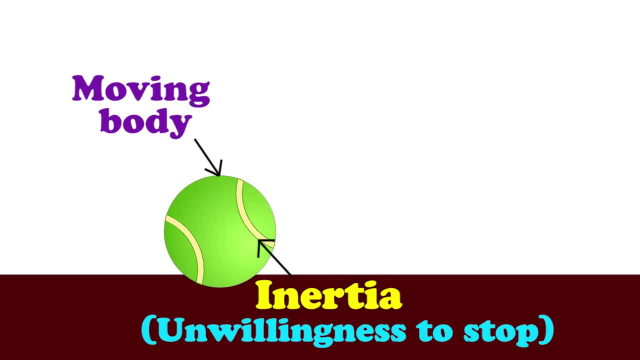 It is the inertia or unwillingness or laziness of a body to change its state of rest or motion. This means if a body moves, it prefers to remain in motion and finds it difficult to stop unless an outside force acts on it. Similarly, when a body is not moving or at rest, 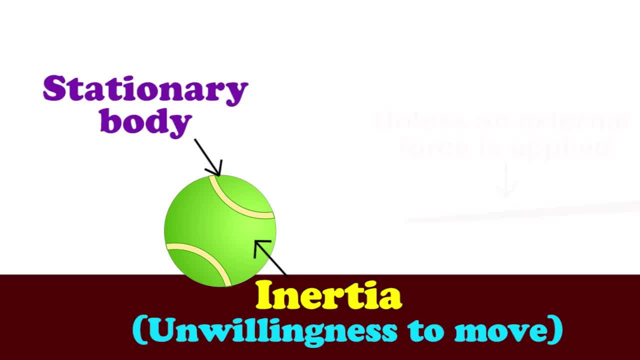 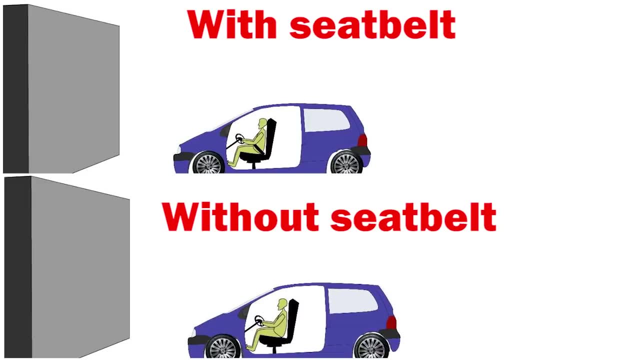 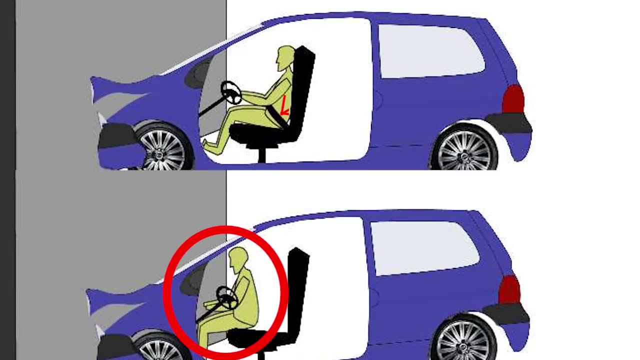 it prefers to stay that way and finds it difficult to start moving unless an outside force acts on it. This property of inertia is important for the automobile industry, while mimicking accidents for safer cars to be manufactured. Thus, physics also involves inertia. 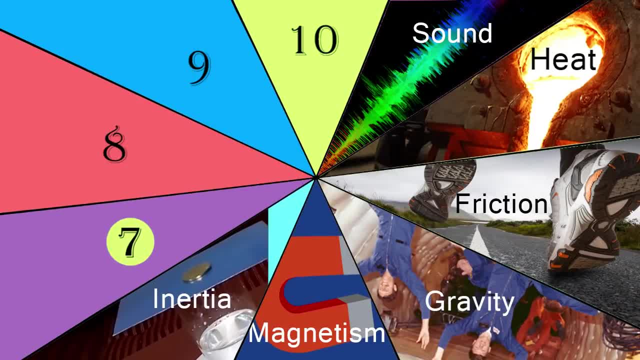 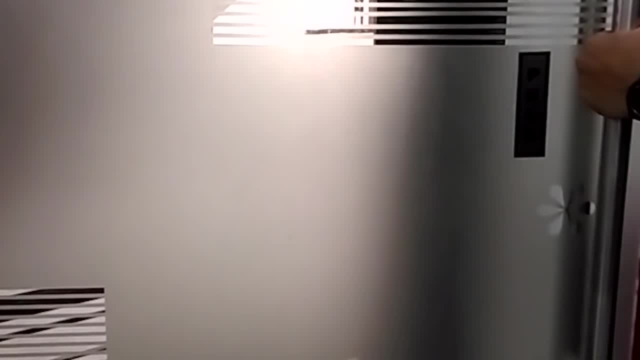 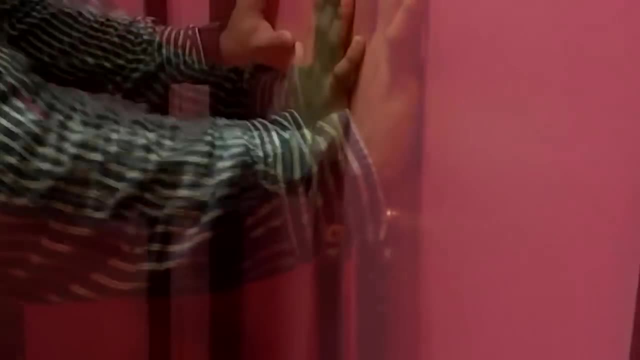 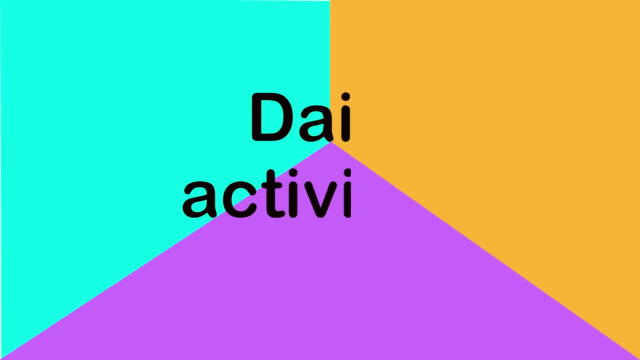 Inertia. Speaking of tugs or pushes, what do we do? when we open or close a door, We use force. When the door is heavy, we use more strength to move it, which simply means that we use more force. Force is something that we use on a daily basis in almost all tasks we undertake, like brushing our teeth, pushing buttons on a keyboard or cell phone. 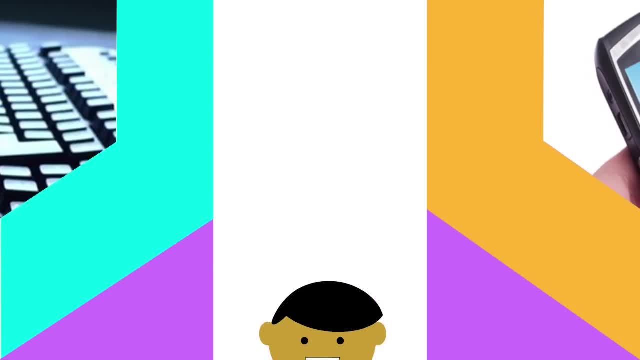 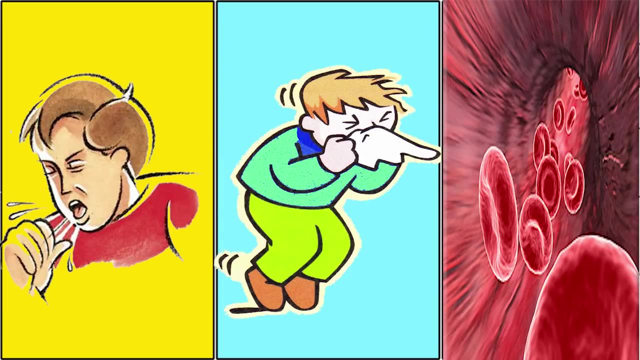 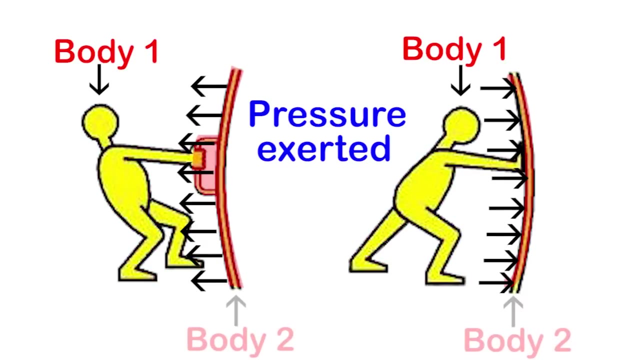 Force is also involved in various processes like coughing, sneezing and blood flow due to the contraction of certain muscles in our body. Simply put, force is nothing but the pressure exerted by one body on another body Sports like swimming or running also employ force. 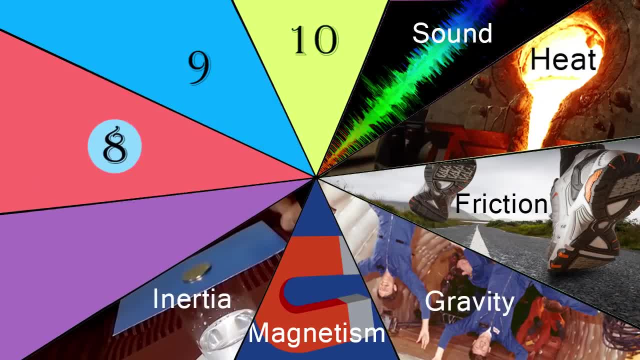 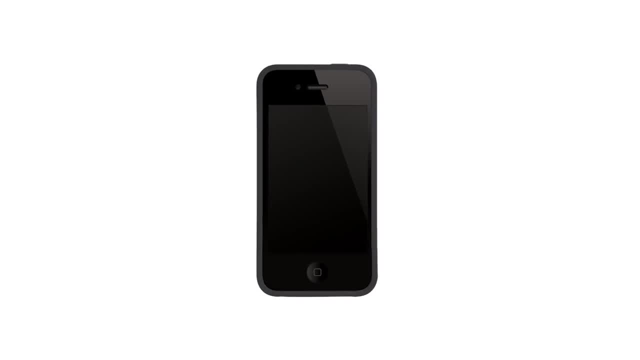 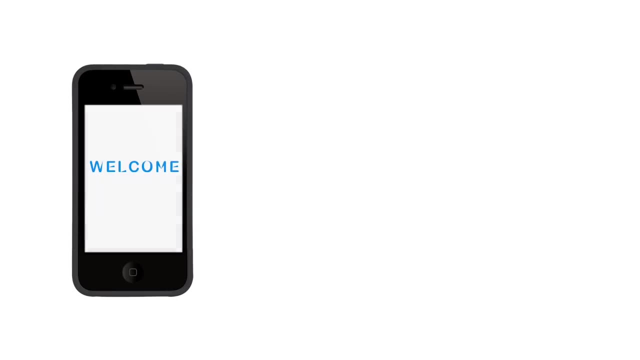 For this reason, force is also dealt with by physics. Let's look into our daily gadgets like the cell phone. What makes the cell phone work is the electricity that's supplied by the battery. What charges the battery is the electricity that's supplied by the power source. 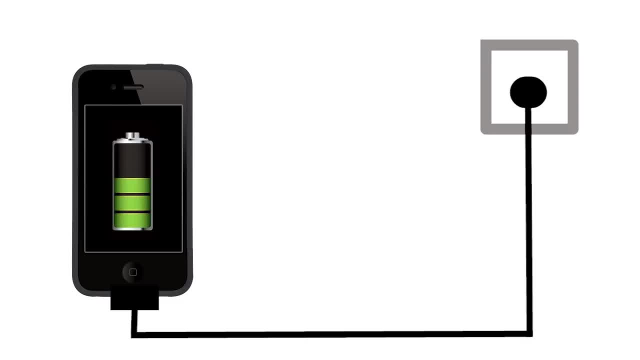 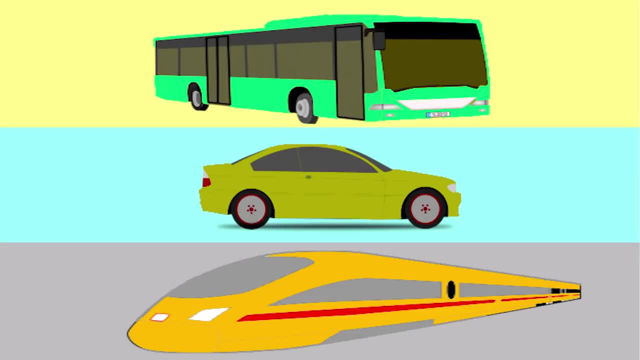 Electricity, as we all know, is an important part of our daily lives, Be it for transportation, like buses, cars or trains, or for powering our household appliances, like the television, the fridge, the microwave, or even to watch this video. 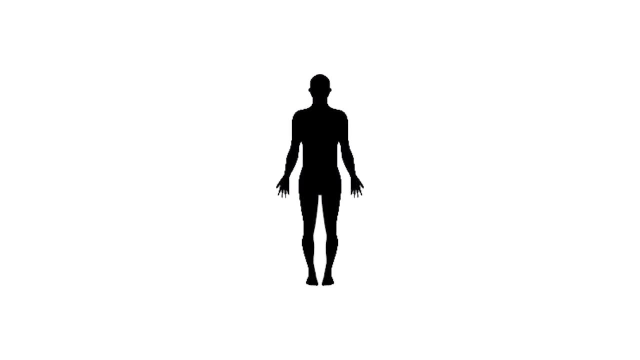 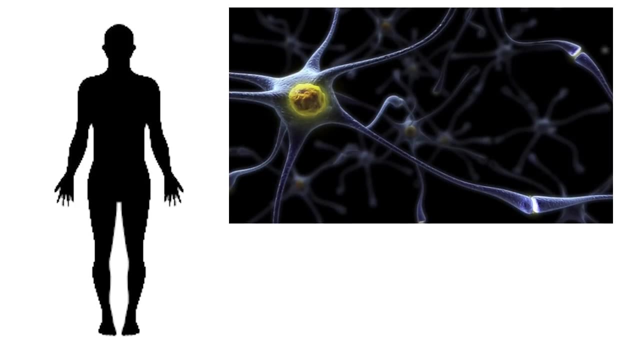 Did you know that our body is also like an appliance and the power to run it comes from certain cells which produce electricity. This type of electricity is called as bioelectricity, which we will see in our biology videos. Though we all are biological systems, the mechanism of electricity production is explained by physics. 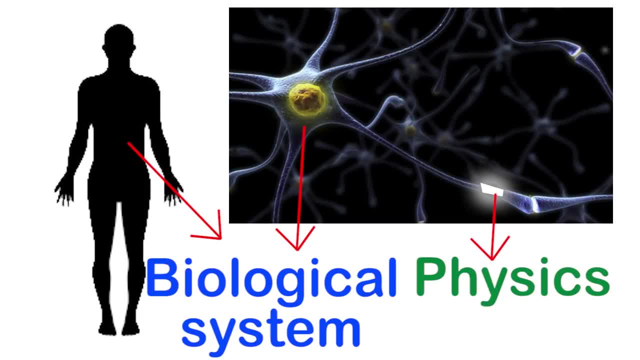 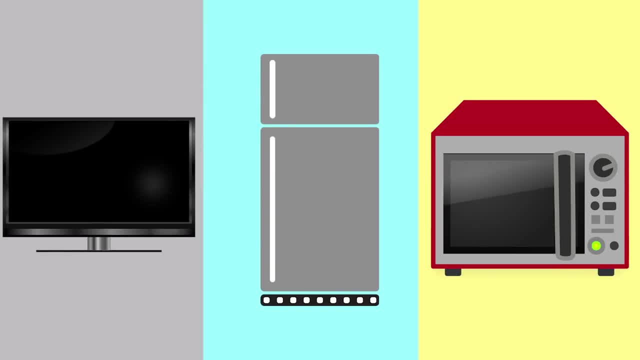 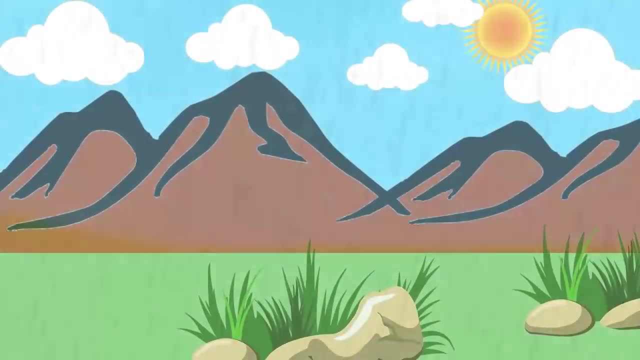 Remember, if electricity can rock your world, it can also shock your world. The many usages of electricity is enough proof to justify why we include electricity in physics. After a while of rain, we see a rainbow in the sky. It is beautiful and has seven different colours. 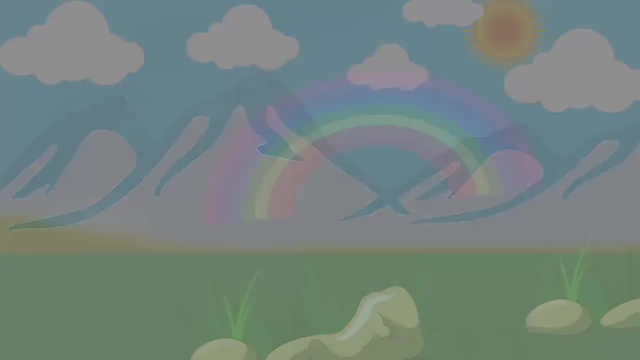 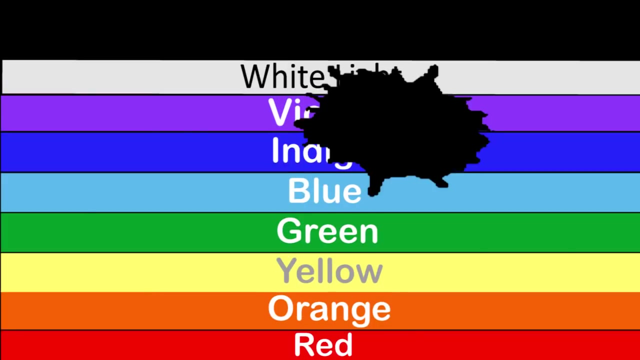 This is a property of light, particularly white light. Though we call it white light, it is actually a mixture of lights of many different colours. Rainbows are formed due to the splitting of sun rays, which is white light through raindrops. 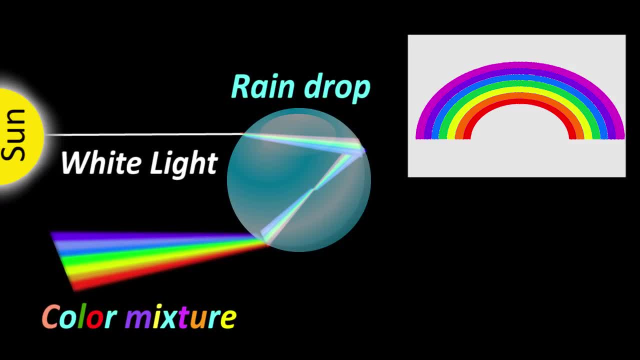 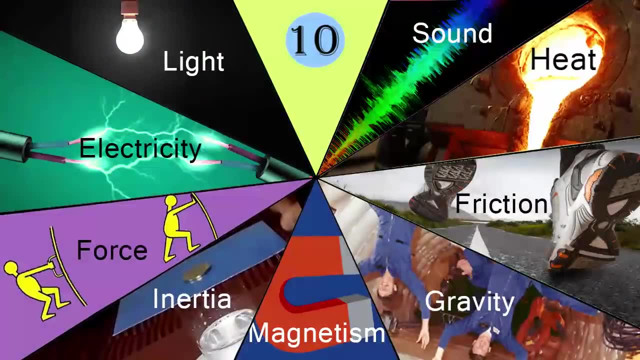 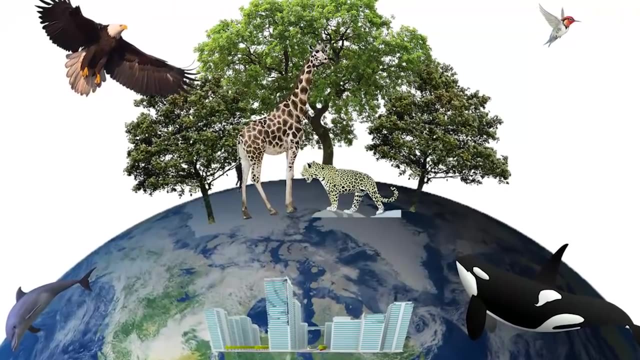 Study of light is an important part of physics because of the various usages of light, like in decorations and lasers. Did you know that we are all made up of many, many smaller particles which we cannot see individually with our naked eyes or even with a microscope? 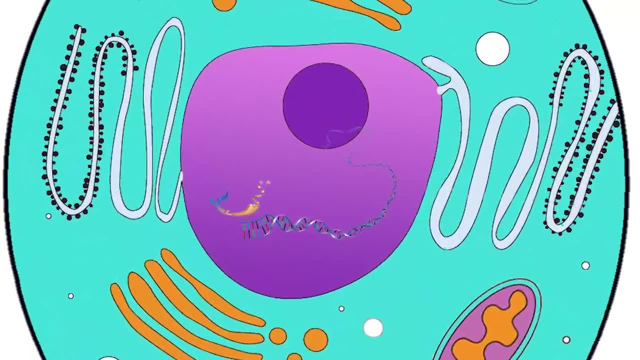 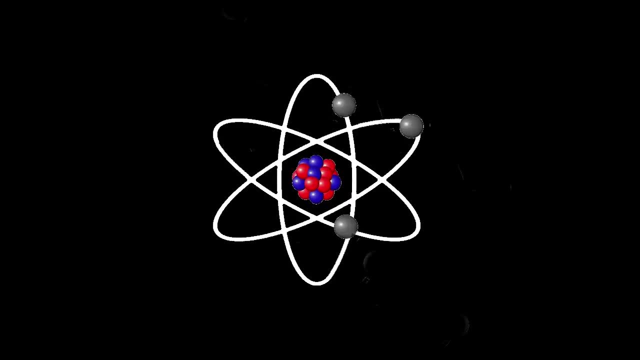 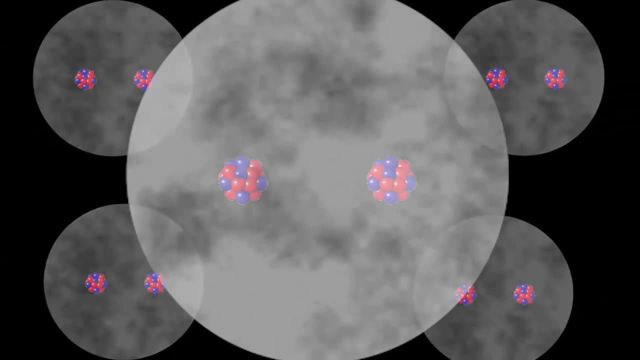 They are even smaller than the smallest cell and in fact these are the very building blocks of cells and everything in the universe. Do you know what these particles are? They are called atoms. Two or more atoms come together to form a molecule, and many molecules come together to form visible matter. 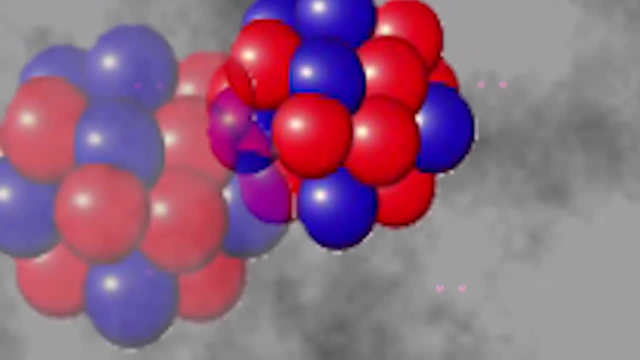 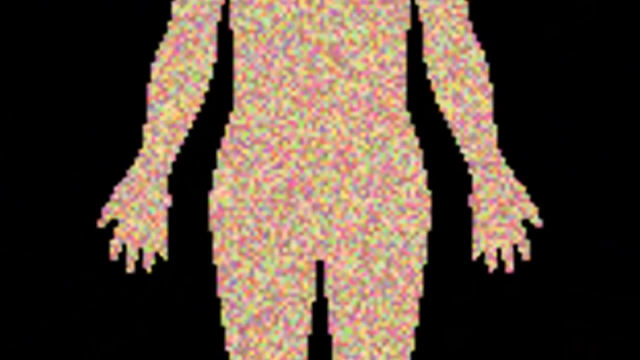 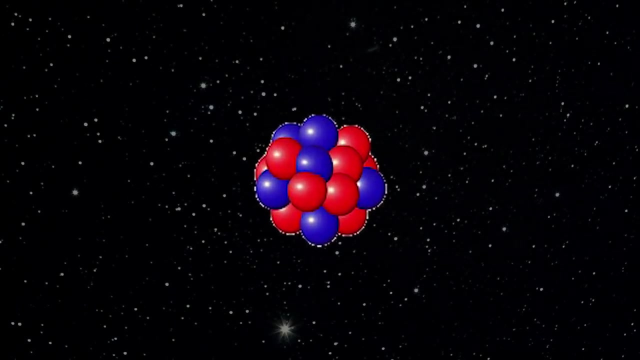 Just imagine how many molecules, and consequently how many more atoms, we are made up of: Billions, trillions, zillions. Even things that we can't see, like minute dust particles, are made up of atoms. The theory of atoms and molecules is involved with the origin of the universe, life on earth and everything around us.